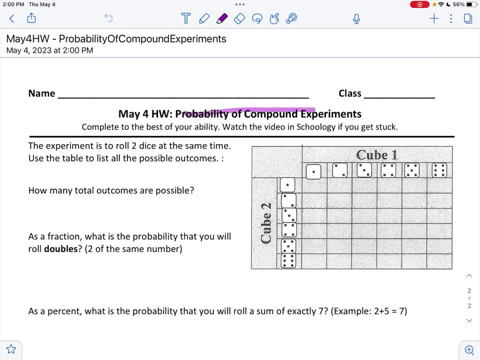 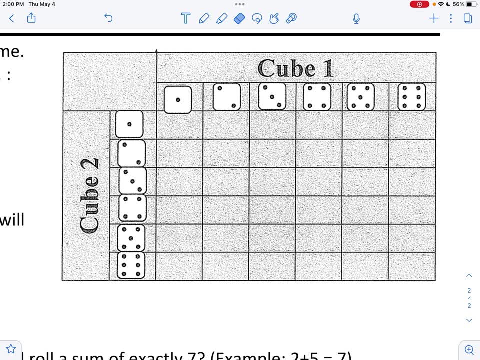 Hello, 6th grade. Today we are working on probability of compound experiments. So down below you can see that there is a table for us to use. It says cube one, so that's dice. This is the first one and this is the other cube right there, Right? so we're going to roll two. 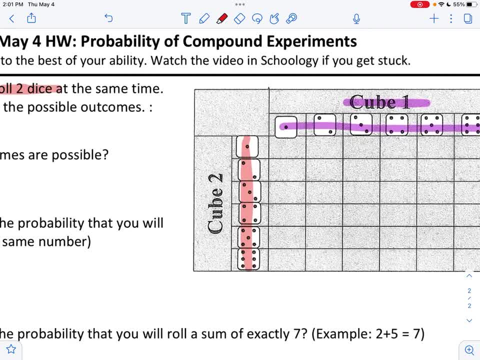 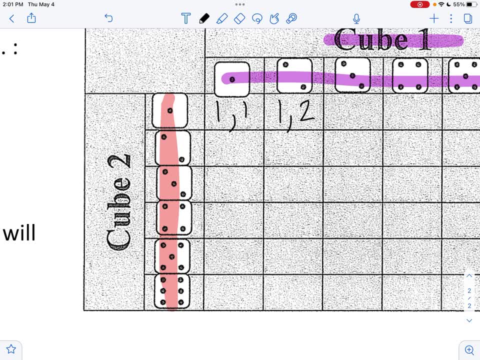 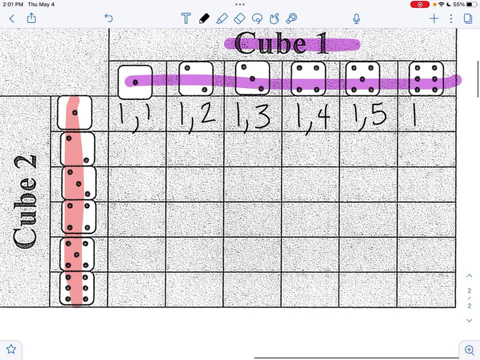 dice at the same time. So something that we could roll would be a one and a one, or we could roll a one and a two, or we could roll a one and a three, or a one and a four, or a one and a five or a one. 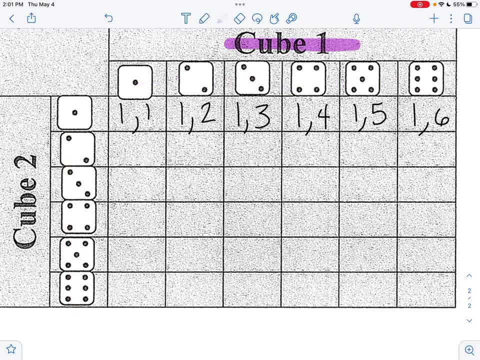 and a six. Okay, so let's back up here, and I want you to see that this one is this one. The first dice could be one and then the second dice could be two dice could be one, or the second dice could be two, or the second dice could be three. 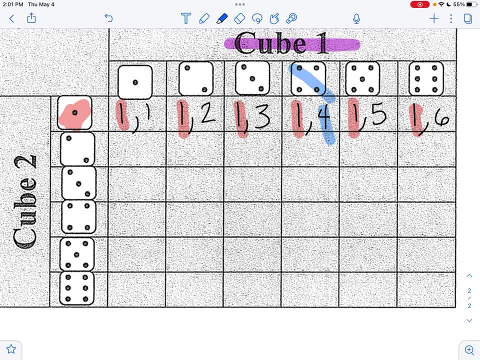 In all of these cases, the first dice always is a one. There's a one and a four, and a one and a five, right? So hopefully you can see where all of that is coming from. Okay, so let's look at the next row. I see that there's a two, so I'm going to write two first. 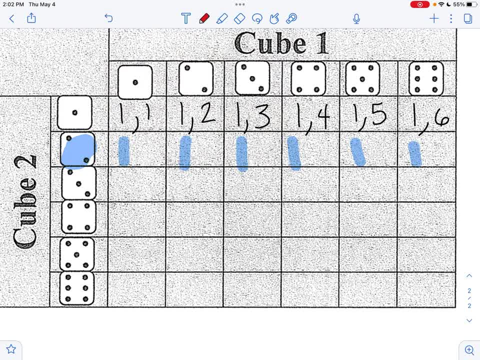 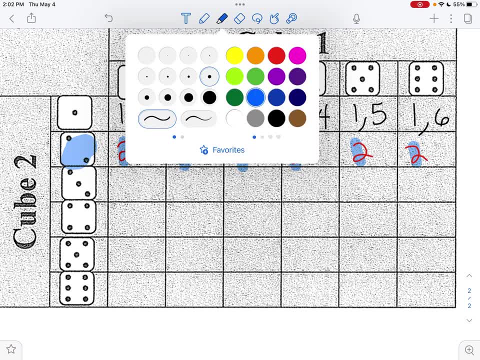 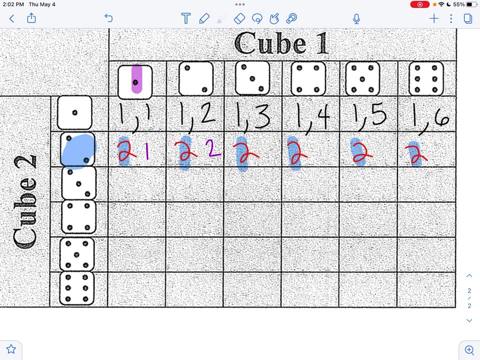 This says that on this roll, instead of getting a one, we got a two with this dice, And then with the other dice, we got a one, and then we got a two, and then we got a three, and then we got a four, and then we got a five, and then we rolled a six. 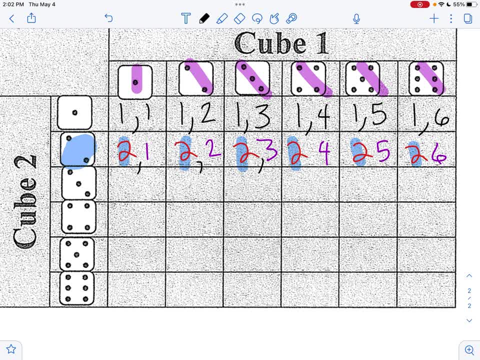 I'll put a comment Between here so you can see it again. So again, that's not 21,, 22,, 23,, 24,, 25, and 26.. That's first a two, then a one. 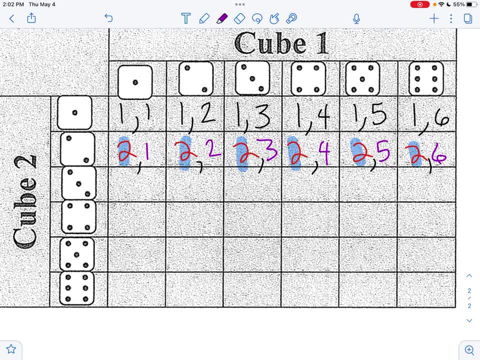 So if we follow this pattern across, we can see that going down is going to be a whole bunch of ones. Going down in this column is going to be a whole bunch of twos, The next one is going to be threes, The one after that is fours, then fives and, following the last, sixes. 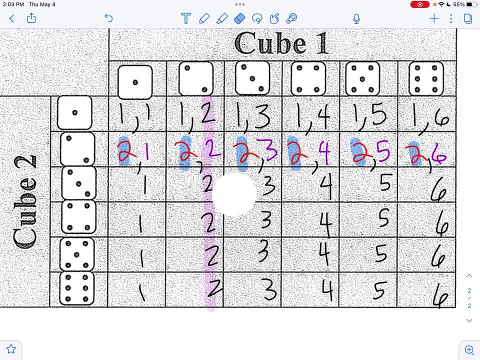 All right, so that's just one dice. Now let's look across at our patterns. So remember how there was a one on top, Then every single one of these started with one. Well, let's look at the next row In front, there's a three. 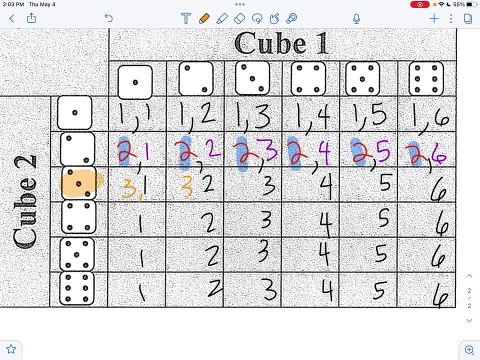 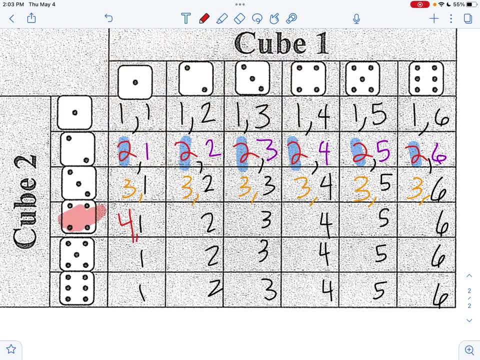 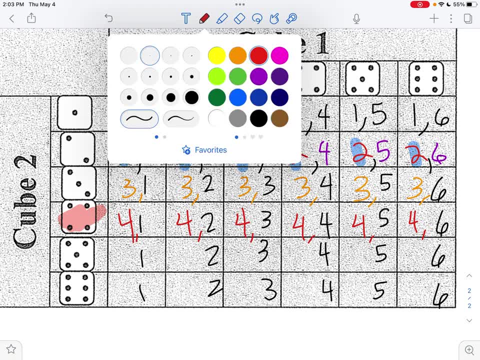 So the first dice lands on four. Four comma one, four comma two, four, four. I think you're catching on to the pattern by now. That means the next one should be five comma five, five, five. 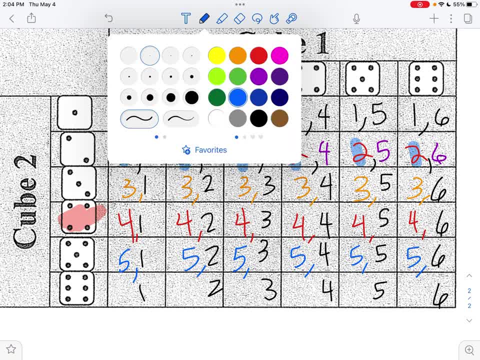 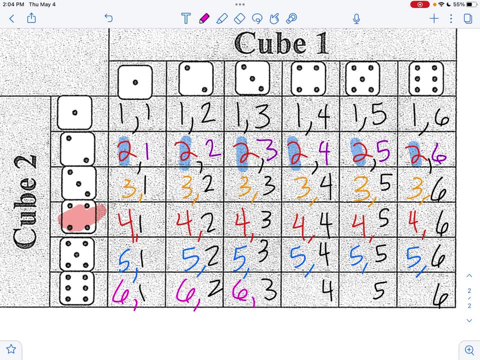 Five, five, and then the last one, we'll use pink. Six comma one, six comma two, six comma three, six comma four, six comma five, six comma six. 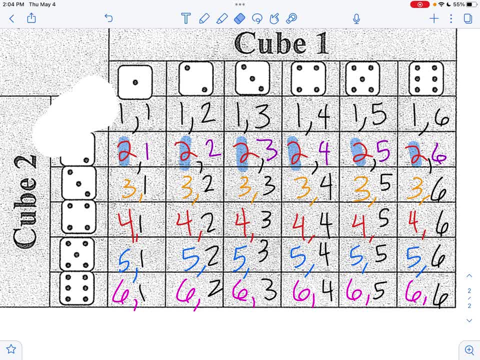 All right, these are all the possible outcomes. I don't know if it'll let me just get the blue, because I wrote the blue first. Oh, it is All right, make this a little bit smaller, then Get the blue. get the blue, get the blue. 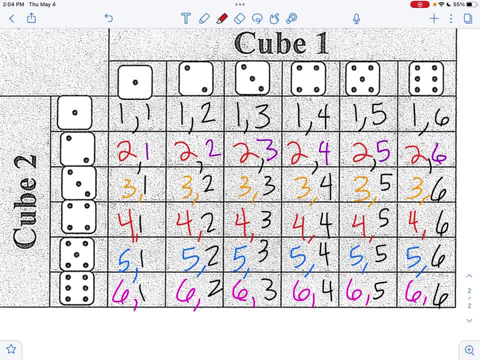 Okay, So where are all of the possible outcomes? We have to include all of them inside this big red rectangle, because all of those have two outcomes. So I can see that it's one, two, three, four, five, six tall and it's one, two, three, four, five, six wide. 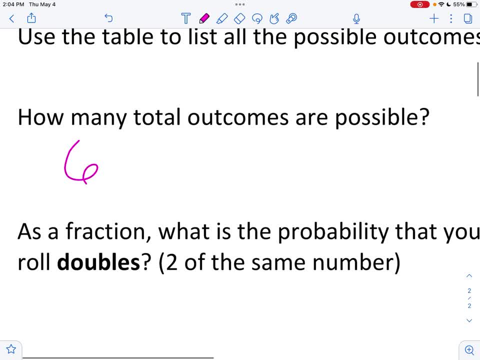 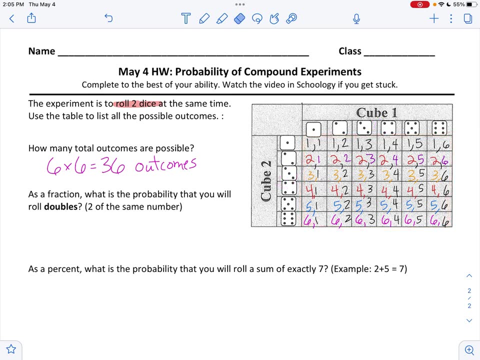 That means for all the possible outcomes. six times six is 36.. 36 outcomes- You can count all of them inside the red. It will be 36.. And if 36 is all the possible outcomes, then for the next couple of problems when it is asking about a fraction. 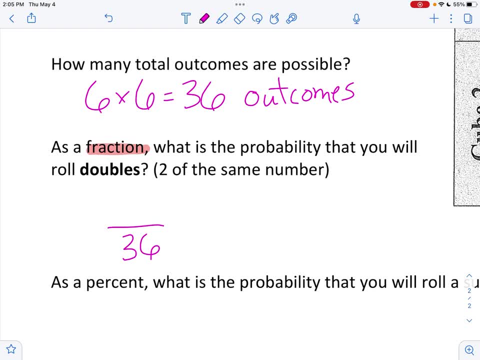 if 36 is all the possible outcomes, then 36 has to be the bottom of the fraction. All right, so now, if I keep reading, it says: what is the probability that you will roll doubles, which is two of the same number. 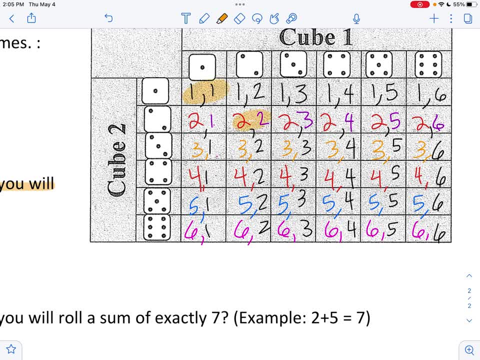 So let's see: Here's a one and a one, Here's a two and a two, Here's a three. Oh, no, Three is not the same as two. Three is not the same as two, So I'm looking for the same number twice. 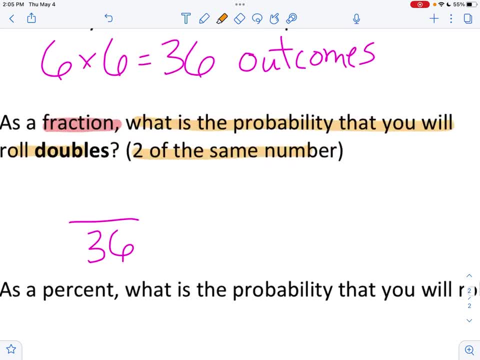 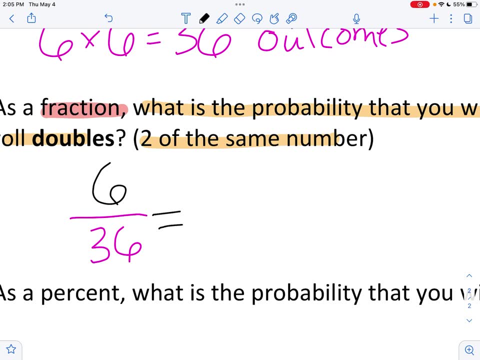 Yeah, cool, A little diagonal line. Looks like there are six, Six out of 36.. And if you want extra credit on your quiz tomorrow, you can simplify this by dividing both of them by six. Divide by six, Divide by six. 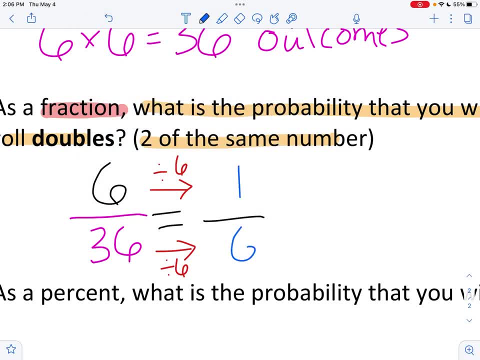 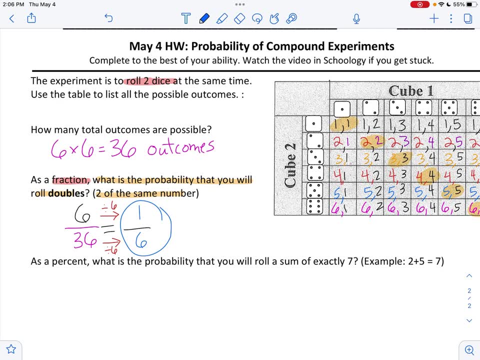 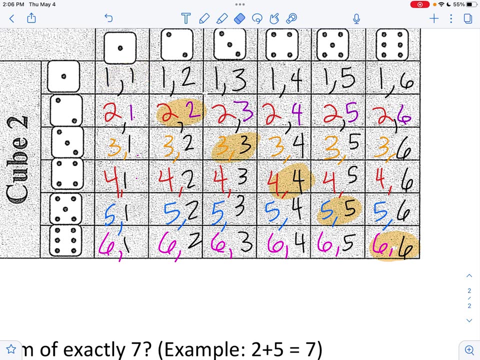 Divide by six Gets us to one sixth. This is the fraction. If we rolled six times, we would expect that one of those times we would get doubles. Okay, let's get rid of this now. Okay, Get rid of the highlighting so it doesn't distract me on the next one. 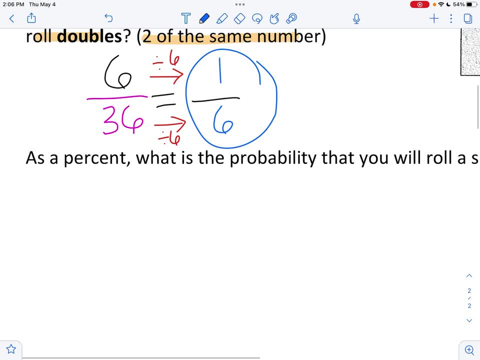 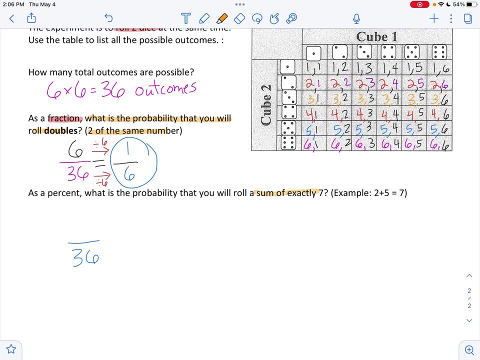 Okay. Next one says as a percent, but I'm going to start with a fraction, And again there's 36 outcomes. What is the probability that you will roll a sum of examples? Exactly seven. So our example is two plus five. 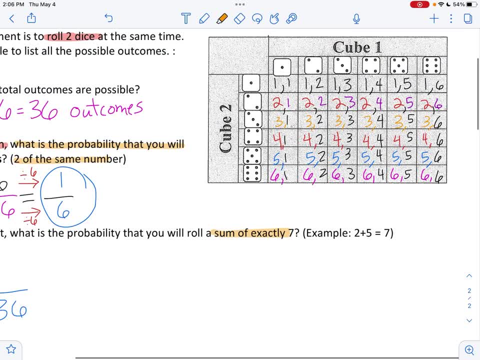 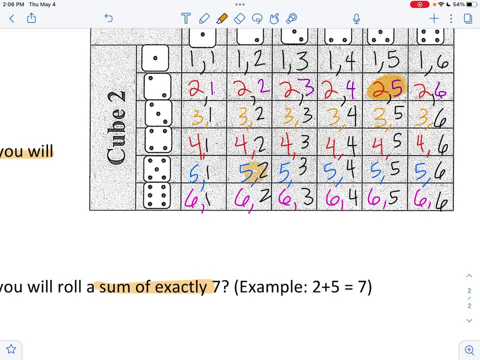 So let's find in our grid two and five. Here's two and five. Put an orange for you. But here's also two and five. The order is reversed. but five plus two is seven. So let's think about another way to make seven. 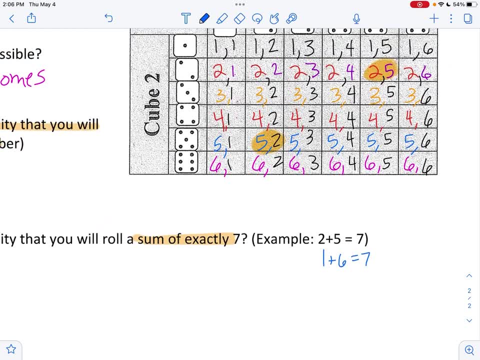 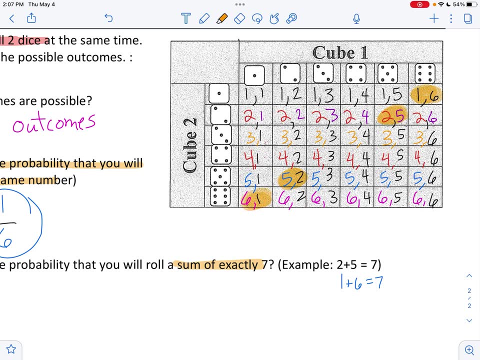 We could say one plus six. So I'm looking for boxes where there's a one and a six. Here's one. Oh, here's one. Okay, Let's see Another way to make seven. Let's see, We used one. 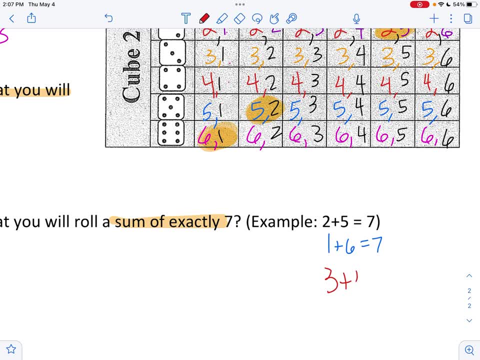 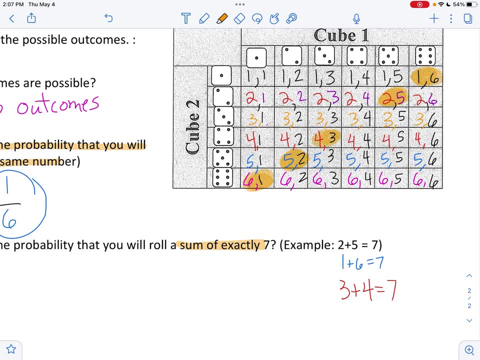 We used two, Let's use three. Three plus four equals seven. So I'm looking for a three and a four. There's a four and a three. That's seven. That's three and a four. That's seven. I think that's it. 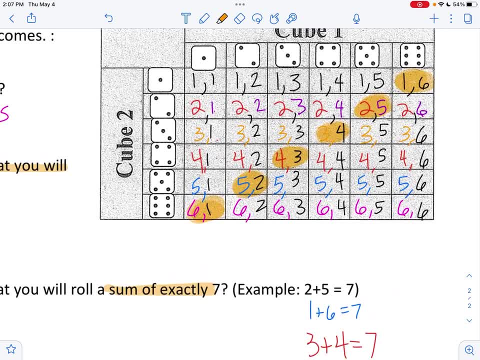 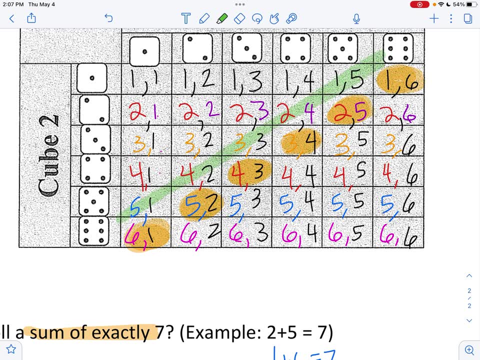 Hey, do you see that It's diagonal again? All right, So that's kind of cool. Let's look and see if there's a pattern here diagonally. I'm going to do kind of this green one here As we go across. it looks like these numbers add up to six. 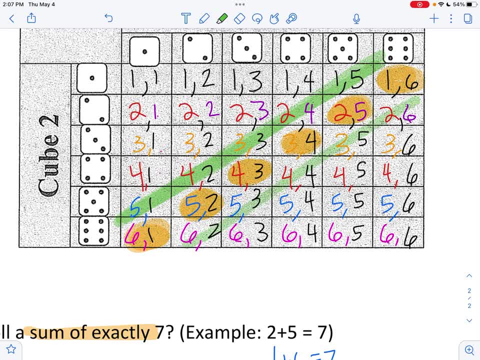 One plus five is six, Two plus four is six, Three plus three, And if you look at this one, they add up to eight, Six plus two, five plus three, four plus four. Let's try another one. This is the nine sum.